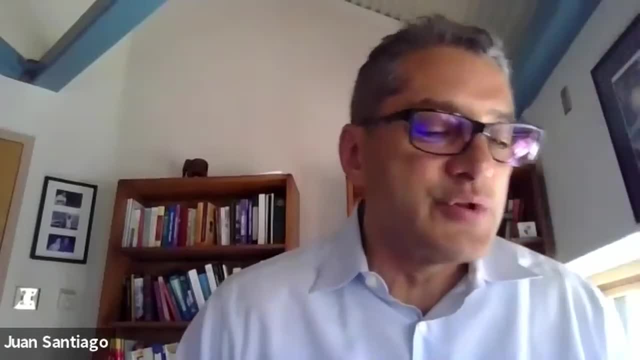 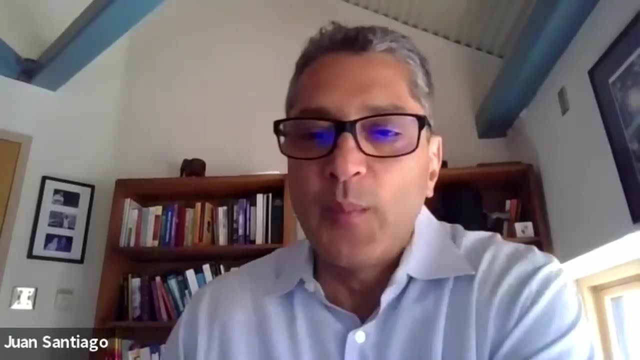 He has served as associate editor and review of geophysics and associate editor of the Journal of Climate. He's authored over 200 papers and we're happy to have him here today. Thanks, Juan, Thank you everybody for joining, whichever time zone you're in. 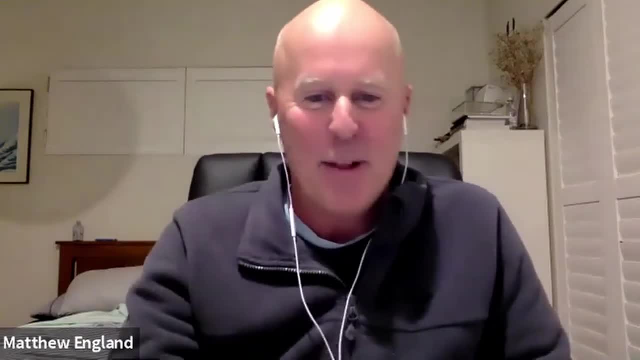 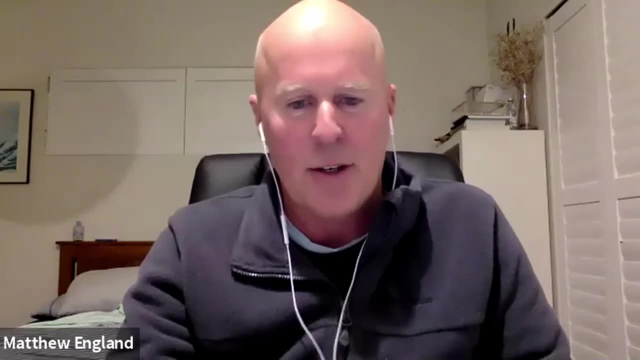 I'm in one that's particularly late at night, about one in the morning here in Australia- but I was really keen to join. It didn't really matter the time for me, I just wanted to join in support of this exciting new journal. 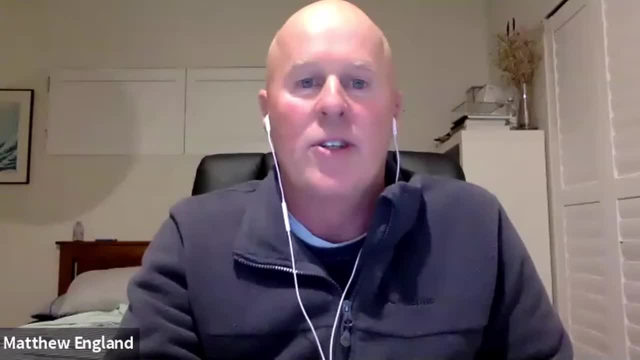 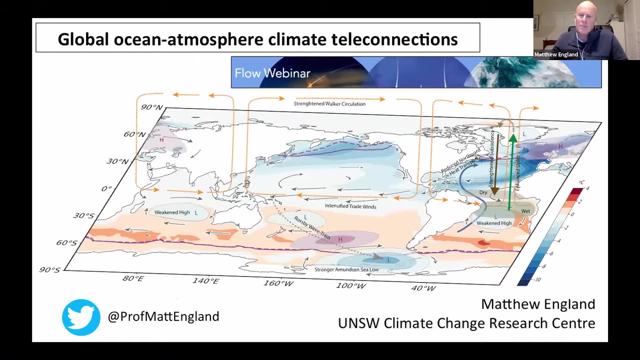 I'm going to share my screen. So, yeah, it's great to join And, as Juan explained, my field in terms of fluid dynamics and fluid mechanics is related to the Earth's climate system- I guess two of the biggest bodies of fluid on Earth- 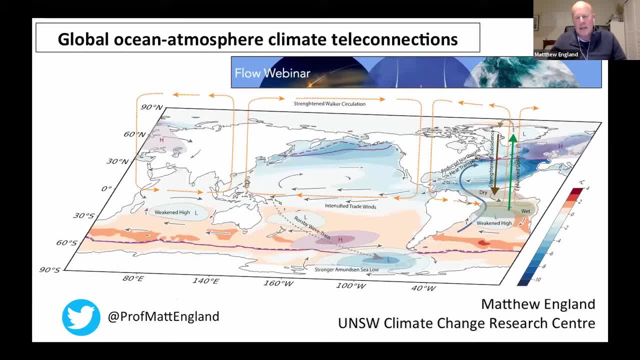 Are the atmosphere in the ocean, and my work's all about understanding the dynamics of these two systems, along with the ice that flows off the ice sheets around Greenland and Antarctica, and the interactions between ice, ocean and atmosphere, How these fluids transport properties around the world when they do so, how it impacts the planet. heat transfer, energy propagation, the uptake of carbon and fluid dynamics underpins all of climate science and all of all of the other things that we do. 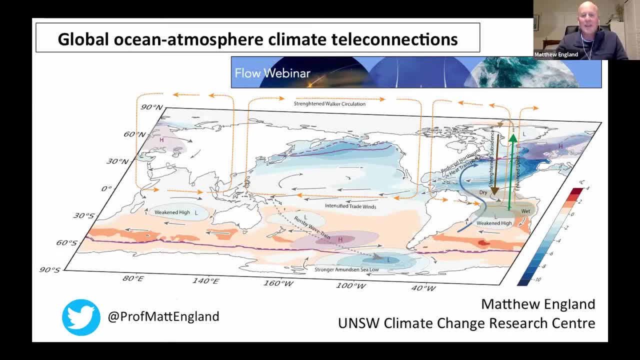 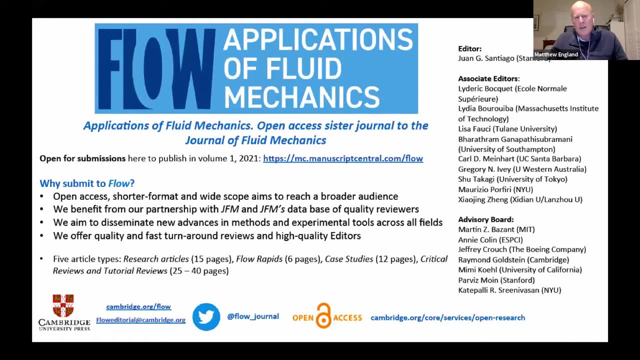 Weather scale, meteorology and oceanography as well. So it's great to be here And before I get into some of my science, I just wanted to give a real plug for this journal. We've we've loved the Journal of Fluid Mechanics for a long time, but I think this new format is very exciting. 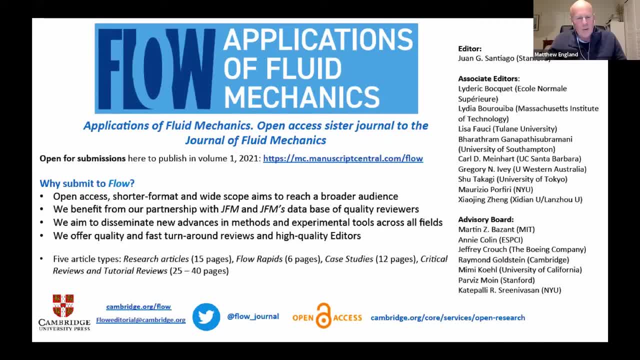 So I wanted to sort of congratulate the team on putting this together. I look forward to reading articles that come, come through and appear And yeah, as I said, as a climate scientist, I'm really pleased to see this, because we can't understand climate change. 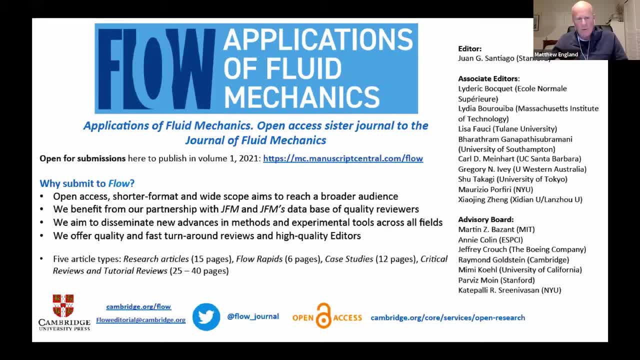 Whether it's climate change or climate change. But I think it's really important to have a deep understanding of the physics of fluid flow in both the ocean and the atmosphere, and of the ice sheets and the interactions between those media and right down to the weather scale. 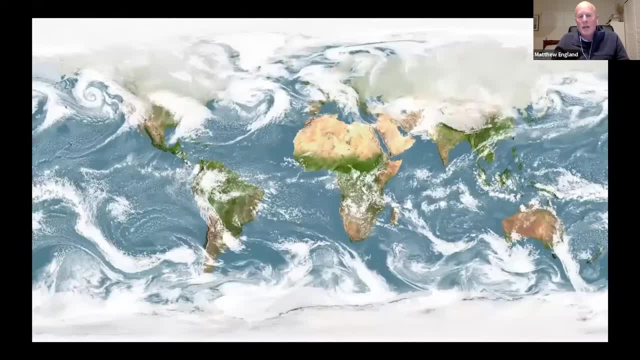 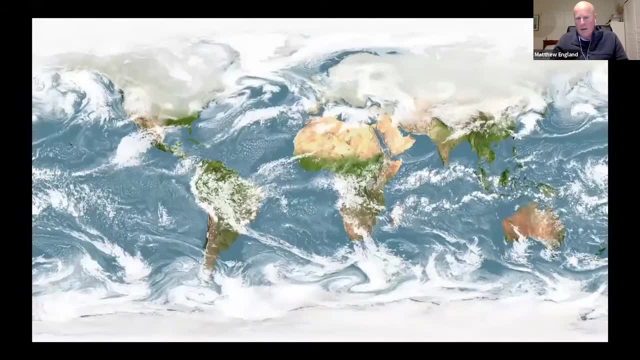 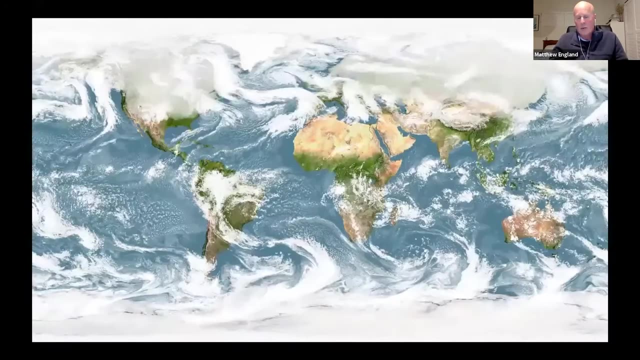 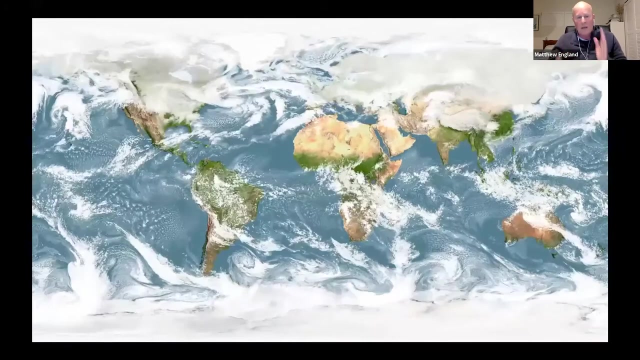 So time scales of seconds through to time scales of millennia. Basically, we live on a fluid covered planet and we're very vulnerable to extremes of weather. We're actually every day. People are affected by the weather they experience, Sometimes in profound And costly ways, with with heat waves and extreme flooding events. here in Australia, it's not long between extreme events. 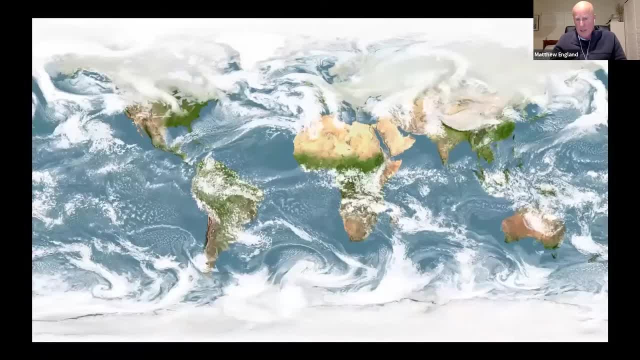 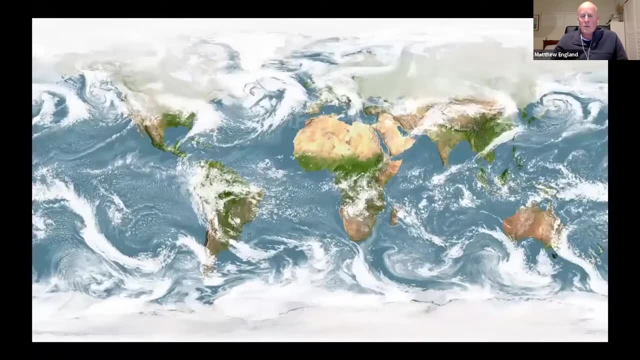 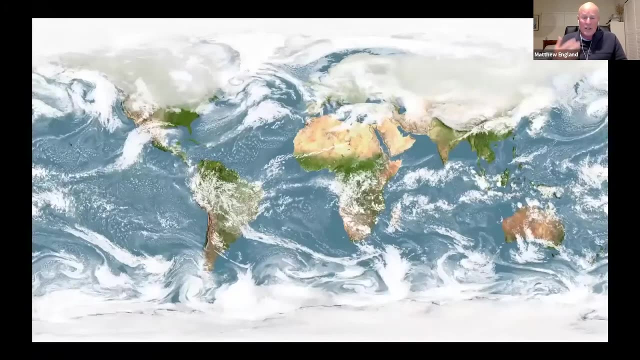 We had a severe flood only a couple of weeks ago in Sydney that did untold damage to the to the coast And we're expecting a lot of these extremes to be to be more prevalent under climate change. But we still are learning some of the dynamics of these systems. the understanding still quite limited. 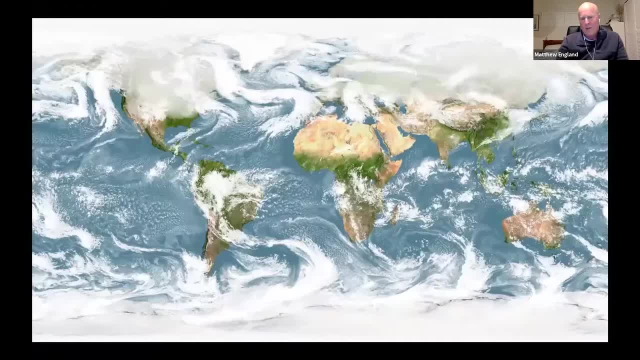 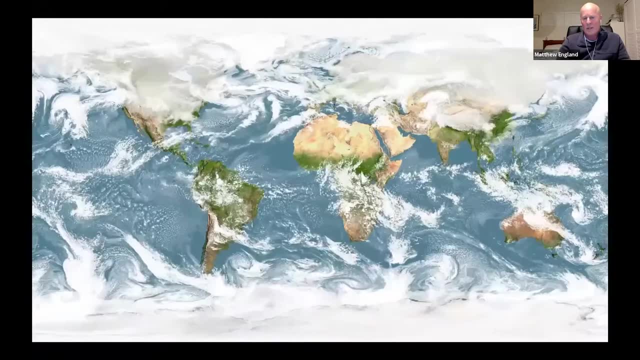 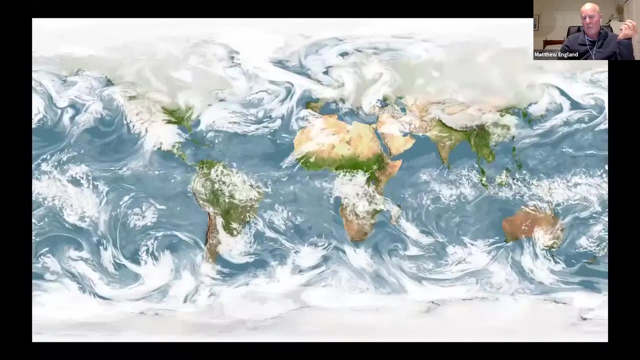 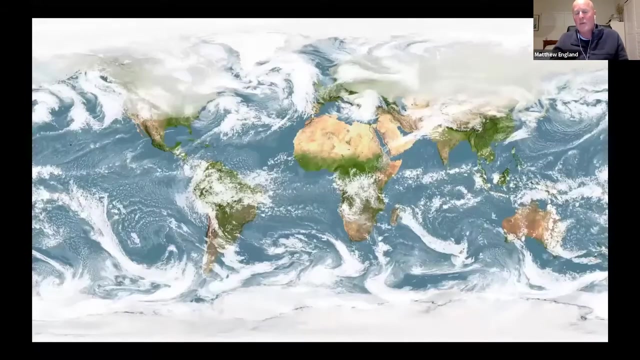 Because our ability to get to the upper reaches of the atmosphere, into the deepest depths of the ocean, is is fundamentally constrained. We don't have nearly enough measurements of parts of these systems, And the other thing is that the fluids, the ocean and the atmosphere, the scales from millimeters and microseconds right through to global scale- there's a cascade of energy across these length and time scales. 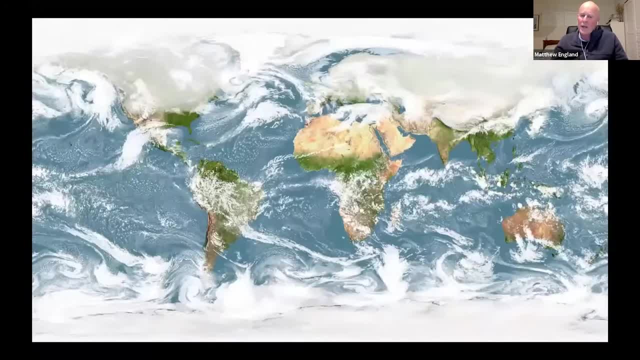 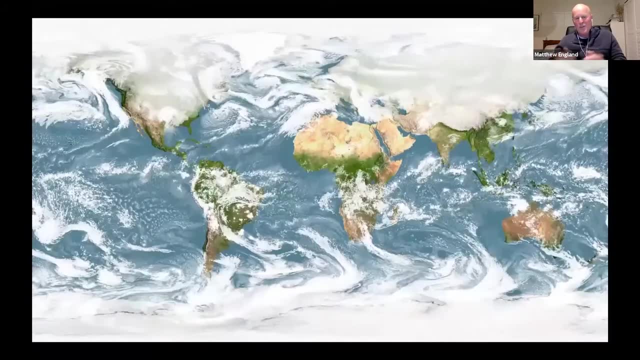 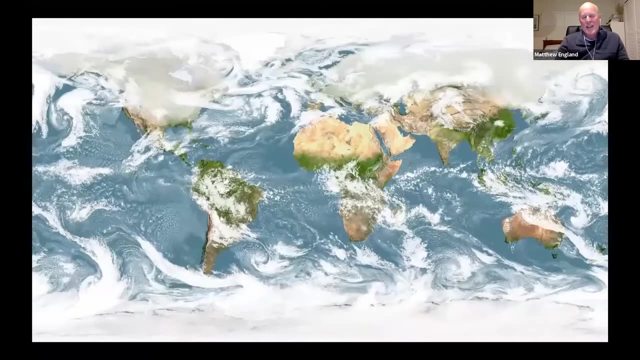 And so, and there's not linear processes too, So it's a complex In a play of processes over order 10 to the 15 magnitude worth of range of time and space scales, if you like. And so that's why there are plenty of us around the planet trying to understand these, these two systems. 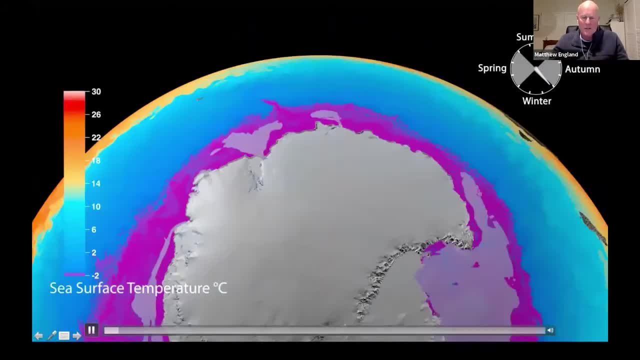 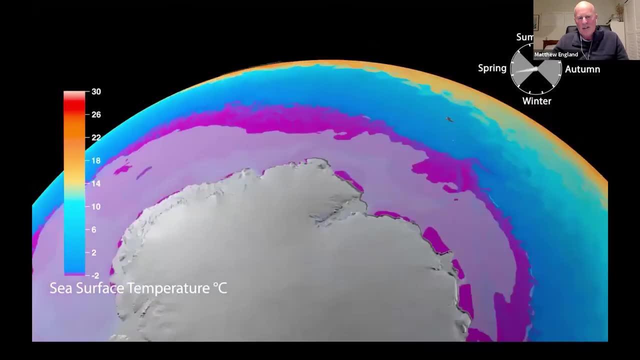 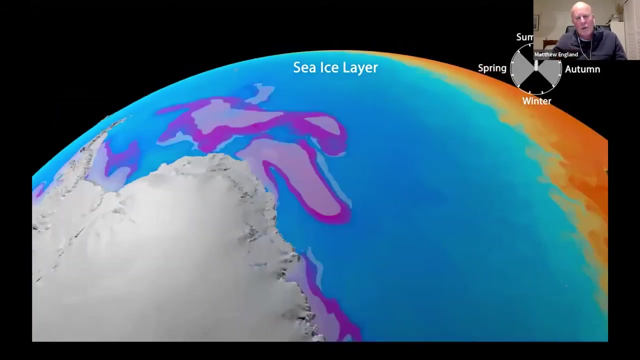 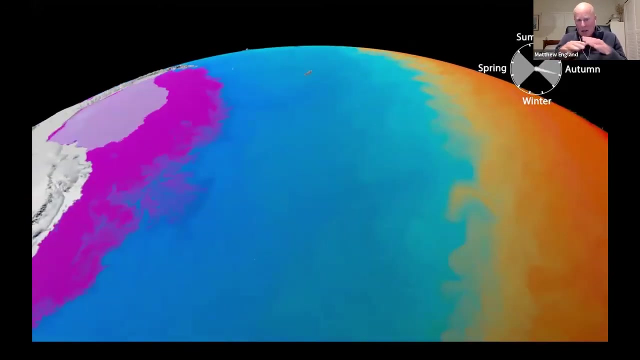 And my, my biggest focus is probably on ocean dynamics. I still see myself more as an oceanographer than an atmospheric scientist, But I also have to say I think the first thing I find about oceans is they are very different, Especially if you look at the ocean. 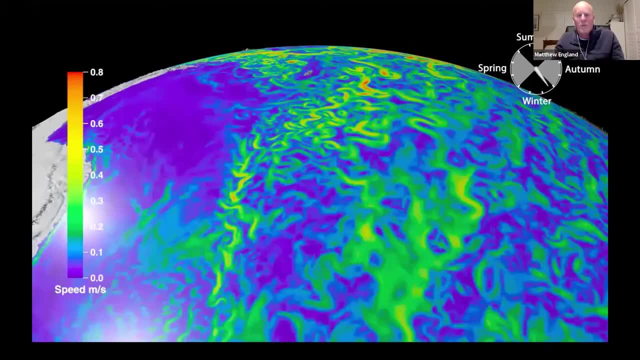 If you look at the ocean, the ocean is a very interesting system, And I think that's something that's really important for us to try and understand. I think that, for the human species, the ocean is our only source of energy, and our only source of energy is the atmosphere. 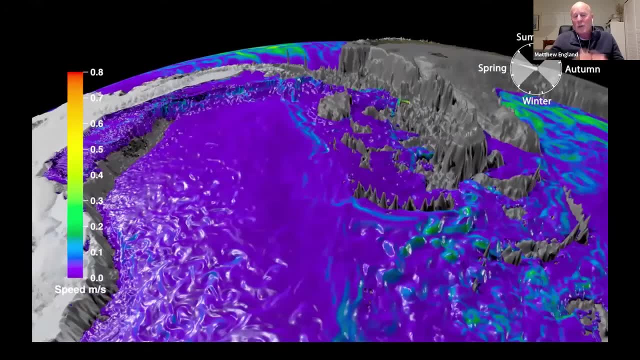 And if it's not energy, we don't know how to do things. So we're not going to know how to solve every problem. We're just going to talk about what happened on a different level. We're not going to get to the deep truth. 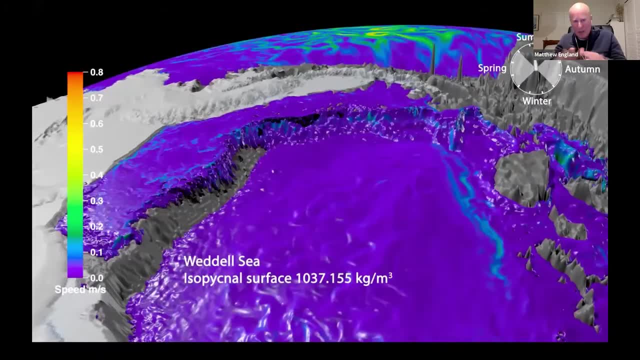 We'll get to some of that, but that's a lot of people's opinion of what happened on a different level, And my guess is that there's going to be an energy shift. There's a lot of different answers: ice caps and so on. this particular animation is showing the fluid flow in the abyssal ocean, so 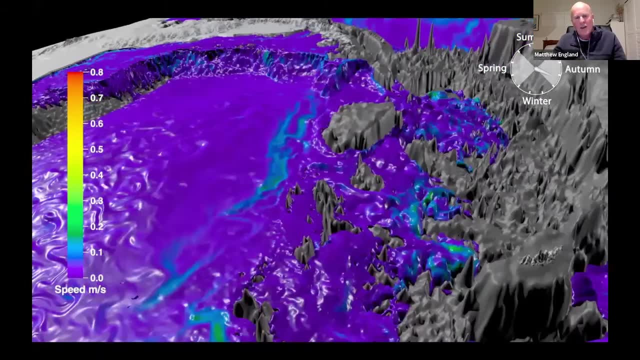 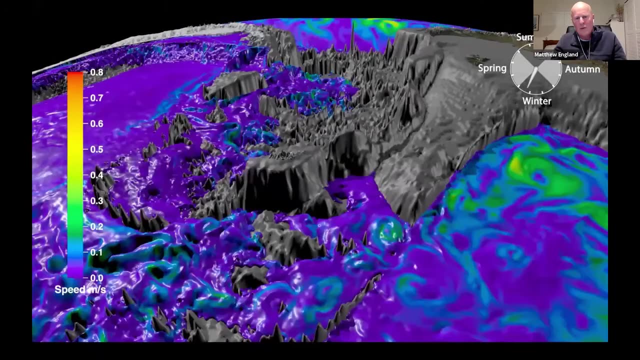 this is the densest classes of water we have. i don't know if it's coming through okay across the internet, whether it's clunky or not, but you can see these um fast flows in in the blues and greens and you can see um filaments of water making their way off the continental shelf. 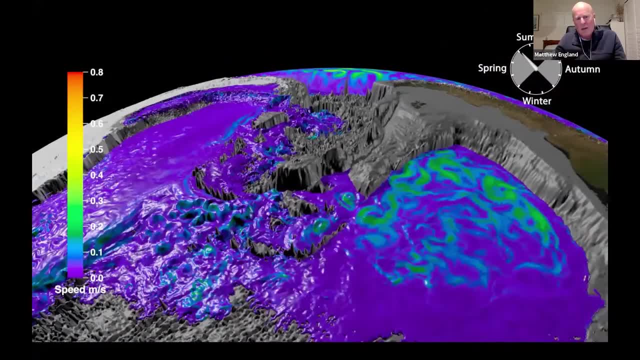 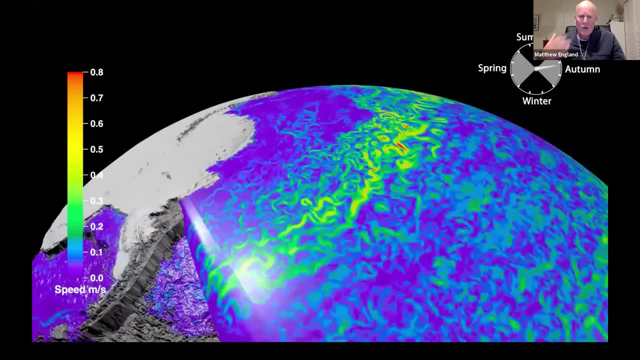 where the densest waters form around autarka and and making, making its way into the abyssal ocean, and this is really important because it, in doing so, it's transporting uh, heat and carbon and nutrients into the bottom of the ocean. this water eventually upwells many hundreds of years later. 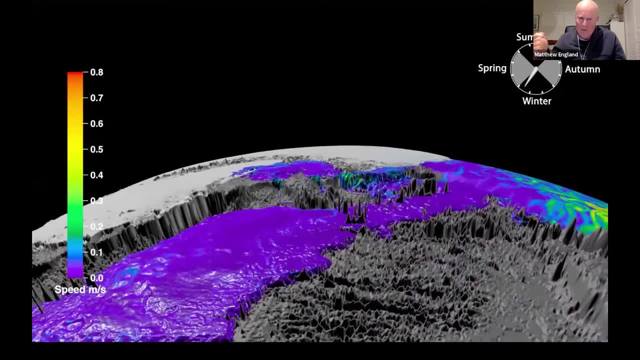 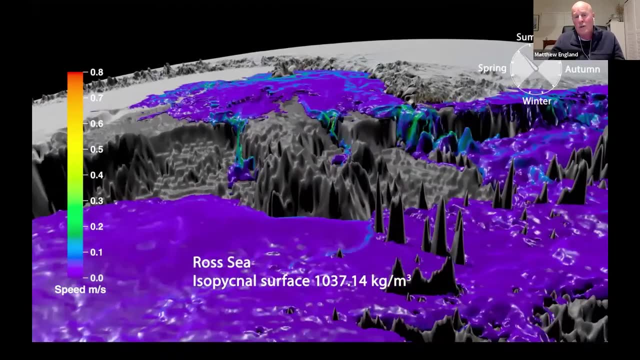 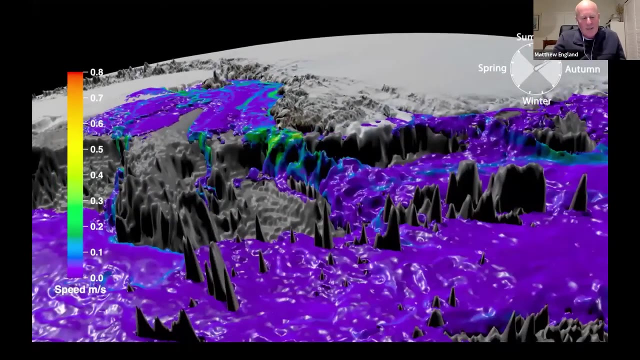 somewhere else. um, and so it. it's, uh, ventilates the ocean and it renews the the ocean of of nutrients and carbon and so on. so it's it's actually critical for for the ecology and ecosystems of the oceans, but it's also critical for regulating our climate system. so that's my 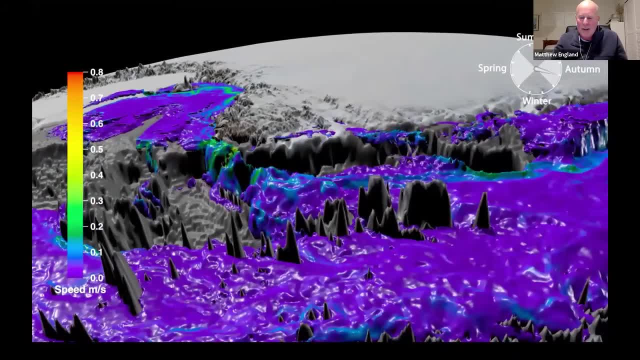 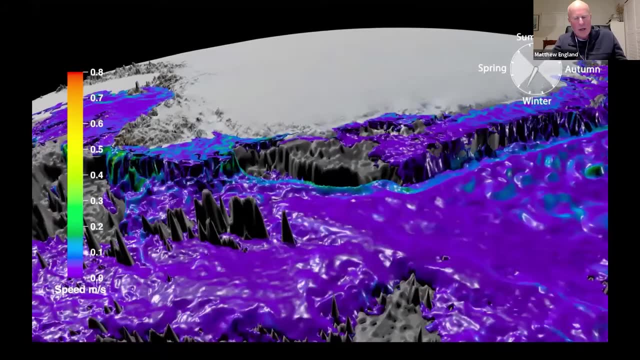 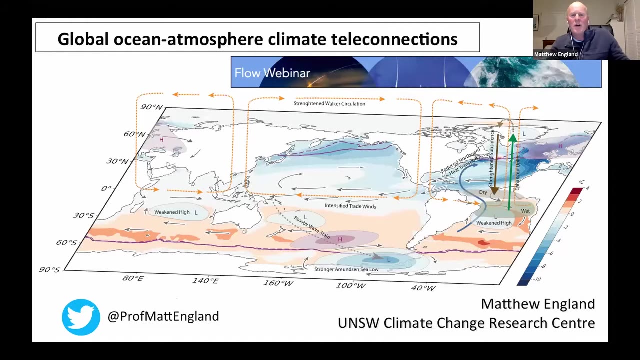 field, and that's why i'm keen about this journal. um, i'm going to get out of the animations for a little bit now and show you some work we've been doing recently on global scale, ocean, atmosphere, climate, teleconnections and- and what i mean by that is i i'm referring to ways that the climate system 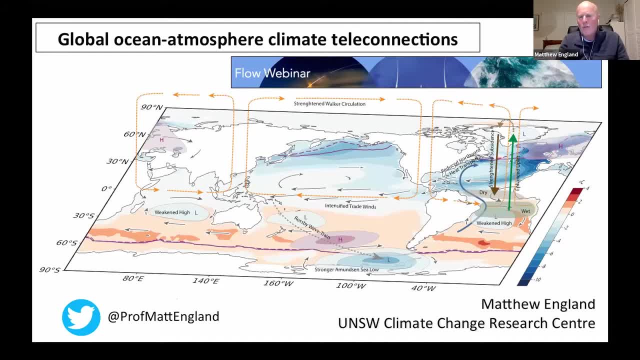 um takes a signal from one bit of uh the planet, maybe say in the north atlantic, here, and and through various dynamical processes, um creates an anomaly or a change in the climate system, sometimes a far distance away, and in this case i'm i'm going to go through how the north 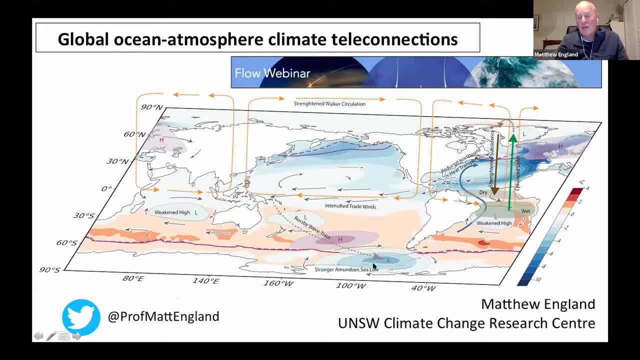 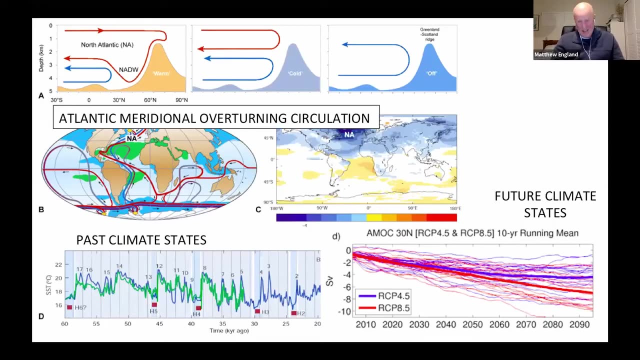 final atlantic. here, um can teleconnect to the, the antarctic here to the far south, and it can do so over relatively fast time scales, and so um i i think the the range of of fields represented in the summer- 180 participants that have tuned in- has got to be very wide, and so i'm i'm sure there are many. 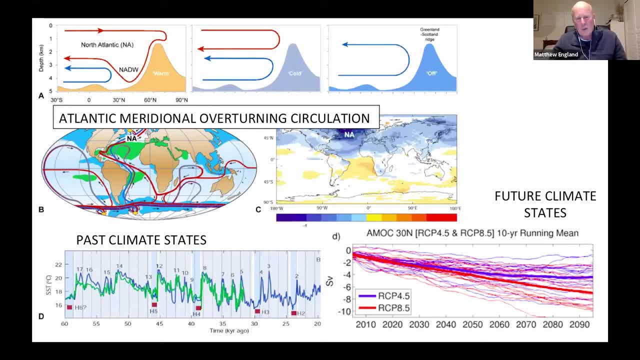 people who haven't heard of this overturning circulation, but i think quite a few would have. it's been popularized in movies even um this massive overturning of heat in the north atlantic, and so, for those of you who haven't heard of this circulation, there's a a flow here into the far. 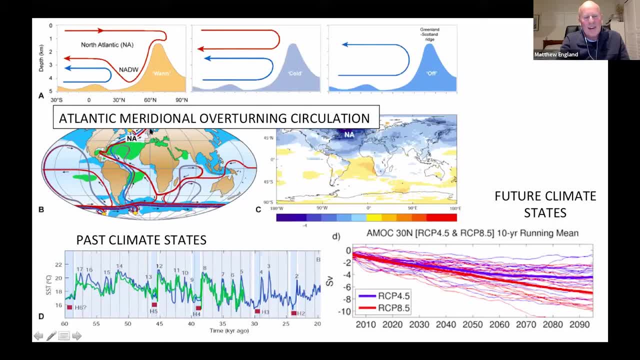 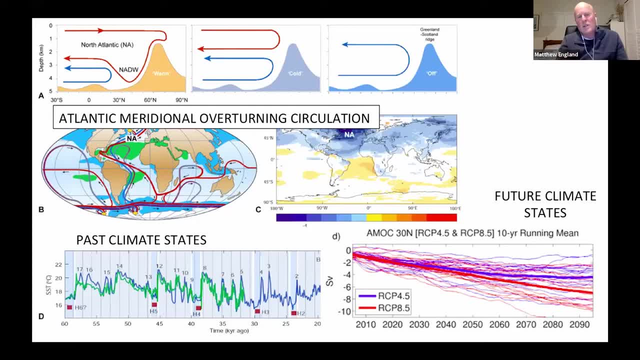 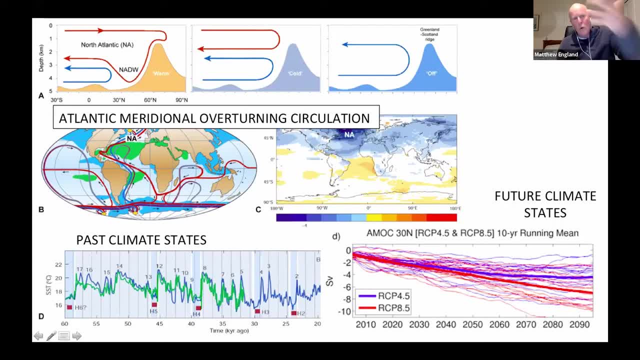 into the deep and abyssal ocean, and in doing so, you know, more water is drawn northward. it's an overturning circulation that's intimately linked to the, the deep water flow, dragging this surface water northward, and in doing so it actually brings a really warm and mild climate to the north. 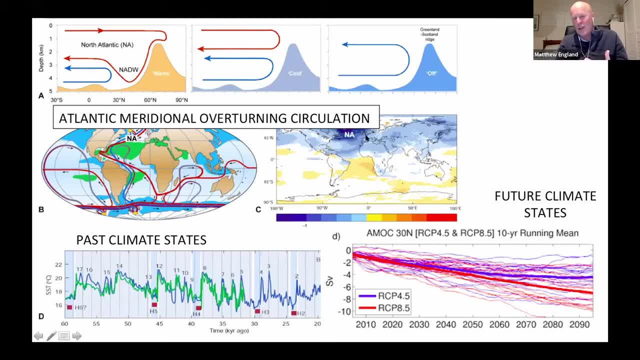 atlantic, and so we're very grateful to this overturning circulation and we're very grateful to this overturning circulation, and we're very grateful to this overturning circulation. it's been what we call on, and and um, and turning over this heat in in today's climate right back. 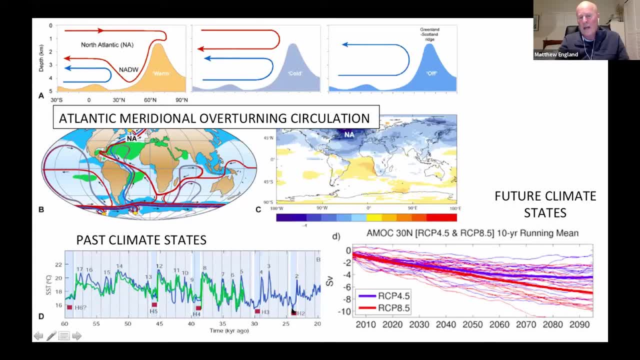 through the holocene. you have to go back to the ice ages for when it actually was last you know, slowed down or off and so um. but there's a lot of concern about this flow because we we know that it it has been off in past climate states and all of our projections going forward. 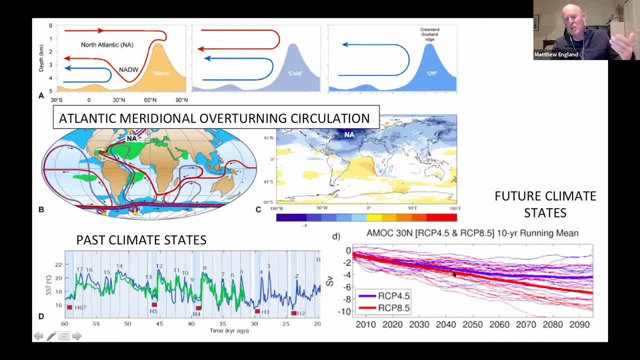 in in the climate change perspective show this circulation to be slowing down. in some simulations it collapses quite rapidly, in others it's more gradual. but we're melting vast amounts of fresh water off Greenland and in doing so we're going to be slowing down the circulation there's. 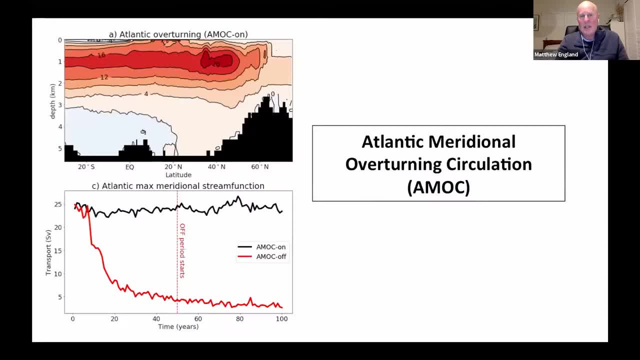 already good evidence of this and and and quite possibly collapsing it. and so the question is: what does this do to the climate system? if we are going to collapse this overturning circulation, what kind of changes will we see outside of the atlantic? and so we did this work with a 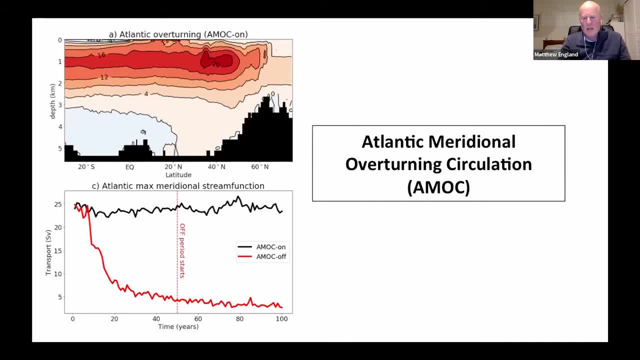 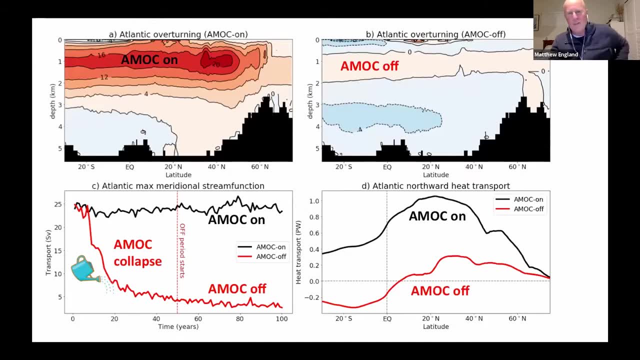 sort of state-of-the-art global coupled climate model and it's, it's simple stuff uh to to do. you can, you can switch off, and maybe that's already confronting in itself the fact that is it is simple to switch off the overturning you. you basically go to one of these full coupled 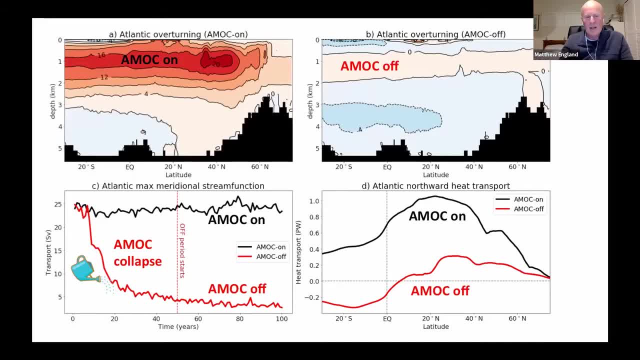 climate models and you, you add some melt water into the north atlantic and that fresh water is less dense and so, pretty much, uh, in short time scales, you, you can cap off the overturning circulation and, um, that leads to, uh, all sorts of changes and the the most obvious changes initially, 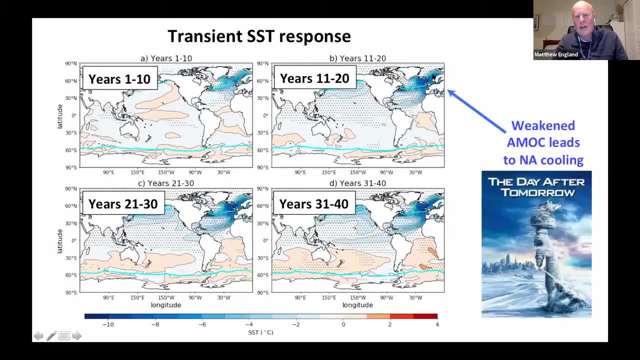 uh, this cooling in the far north atlantic, and i put a little icon here for the for the day after tomorrow, um, because, um, this is the sort of hollywood blockbuster that came along um popularizing this, um overturning circulation and sort of dramatically showing that the shutdown could. 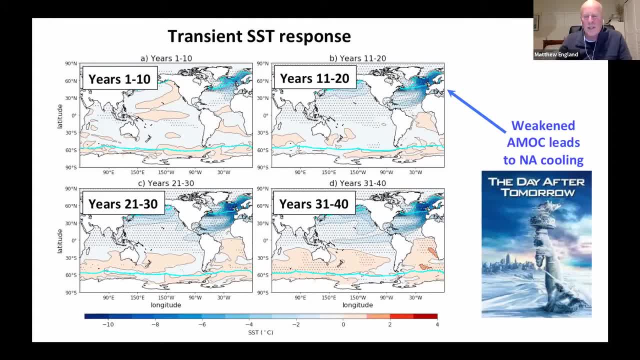 could lead to an ice age within days and- and of course, this was science fiction and completely not what happens in the real system- it takes thousands of years to build up ice sheets. um, but nonetheless it was. it's true that if you shut down the overturning circulation, 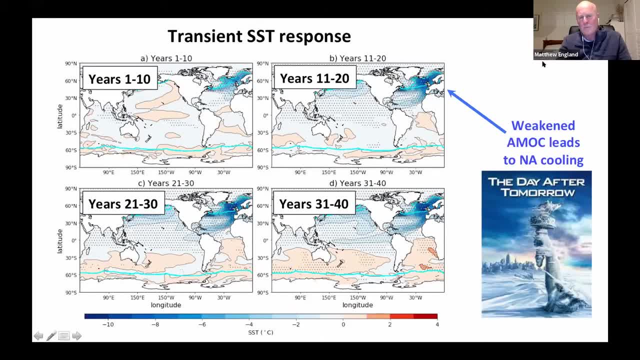 you get a dramatic cooling in the north atlantic and uh, one by the way, please, please, give me some warning of time, uh, because i'm i'm not quite sure where i'm up to in in the in the 15 to 18 minutes i've got. so if you give me a five minute warning, that'd be appreciated, okay, so, um, this cooling, that 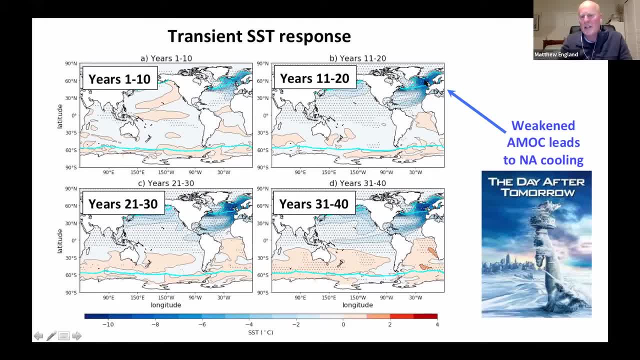 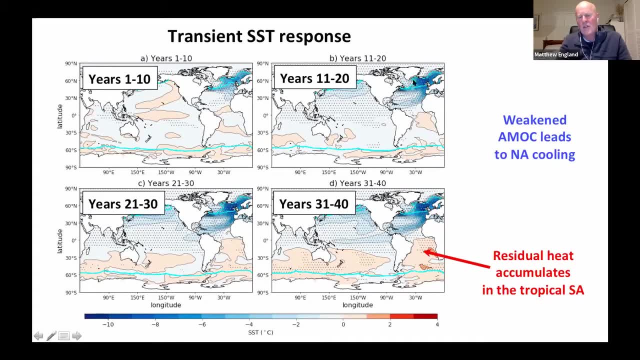 we get has been documented in many, many papers, but much less understood is the teleconnection that goes beyond the atlantic ocean, and so when we slow down the overturning circulation in the north atlantic, what we do um outside of the atlantic is actually leave a massive, uh, new reservoir of heat in the south atlantic, and so this residual heat 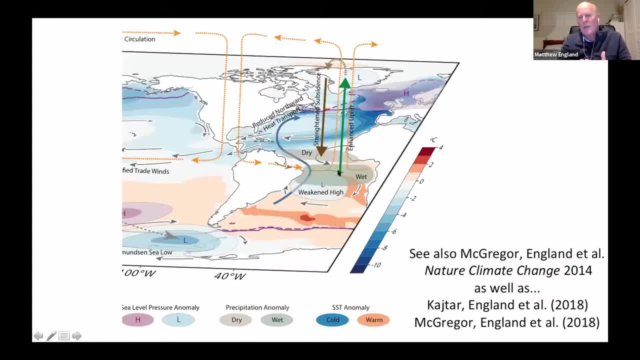 accumulates in the south atlantic, and and then what happens? uh, warmer water leads to warmer air, and that is less dense. it convectively moves up into the upper reaches of the atmosphere, as shown in this cartoon here, and and so you then get a subsidence or a descent of air over the east. 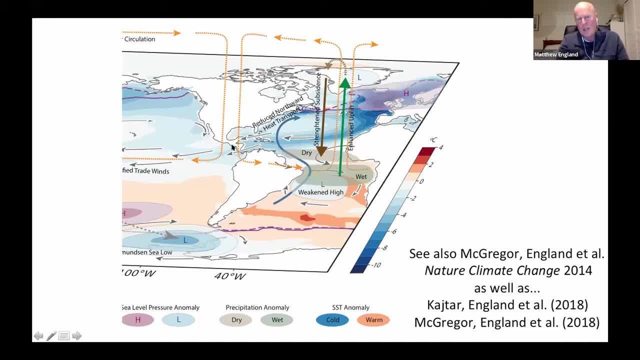 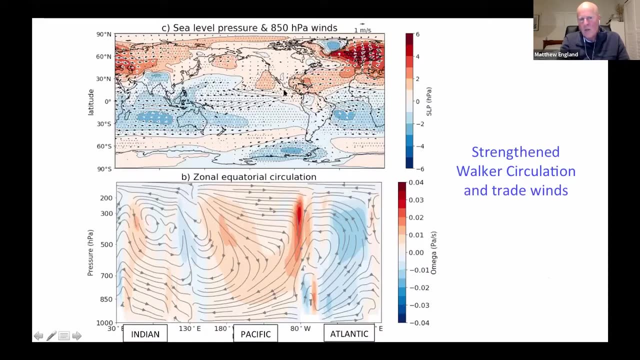 pacific and there's a very important circulation in the east pacific. that's due to these el nino cycles, uh called the walker circulation, and if you start to descend air in the east pacific- here, as i've shown this diagram, you then get an acceleration. so the trade winds here right. 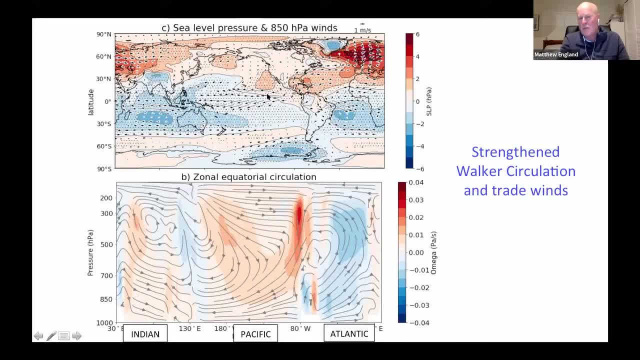 across the pacific ocean in this simulation then become dramatically stronger and this whole walk circulation is now altitude on the on the on the y-axis and longitude along on the x-axis here. so it's a cross-section through the atmosphere going up in height and you can see this overturning. 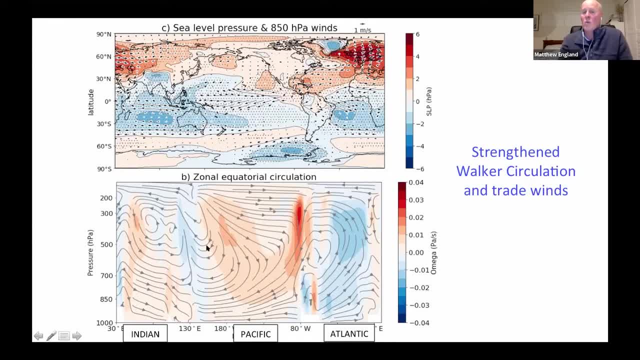 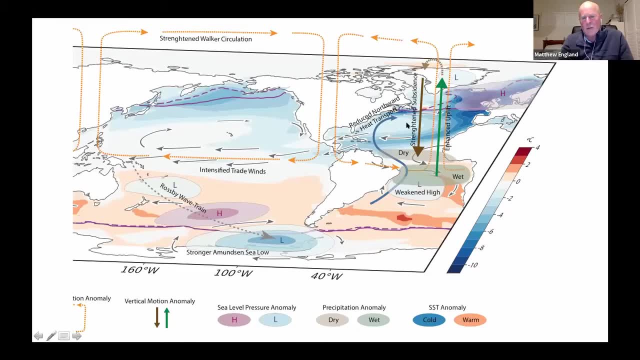 circulation, um the walk, circulation accelerating when we, when we shut down the overturning of the northern lake, deep water, and so we come up with this cartoon diagram- uh, this is under review at nature, climate change at the moment- showing that, uh, this, this slowdown of the overturning, the 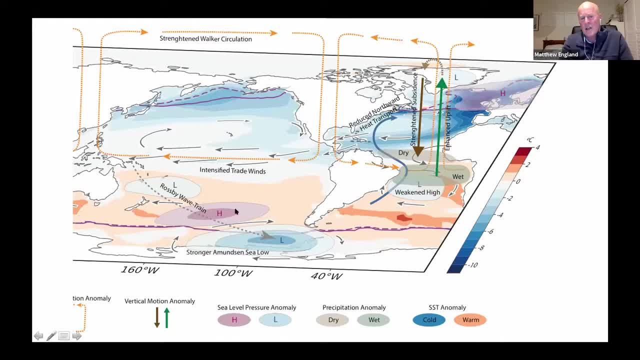 north atlantic actually triggers changes as far as- and how do you see this change? uh, in the north atlantic. so the next slide, please, antarctica. because once you pile up warmer water in the maritime continent region, from these trade winds intensifying, you get, uh, what's known as a rusty wave train. these are waves in the atmosphere. 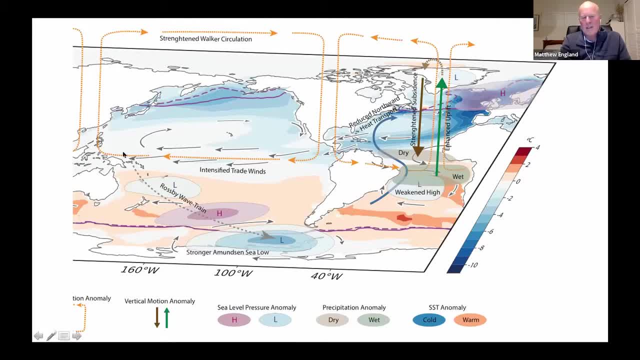 that um uh propagate, uh, that they have a dispersion. i'll go into that in a second. but they, it's basically um the warm air here drives an enhanced hadley cell which is um propagating towards the high latitudes and that disturbs um atmospheric uh, atmospheric uh systems, such that you, you get these waves propagating pole woods with this. 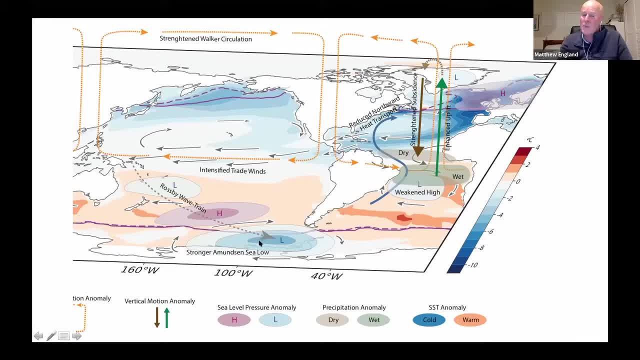 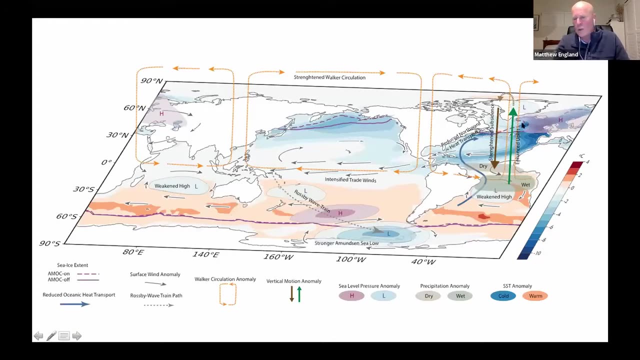 um arc towards the amazon sea region and this, this part of the atmosphere over the last 30 or 40 years has deepened considerably. so this low pressure system here, um off the amazon sea, has deepened considerably. so we put together this summary of what we found, a global scale, to a connection. emanating out of the north atlantic and the, the, the um, the global scale teleconnection emanating out of the north atlantic and the, the, the sending time and oranges andatra along it. what we found response shows it isids Mingtang couldn't do anything. we entered the energy and what we found information. 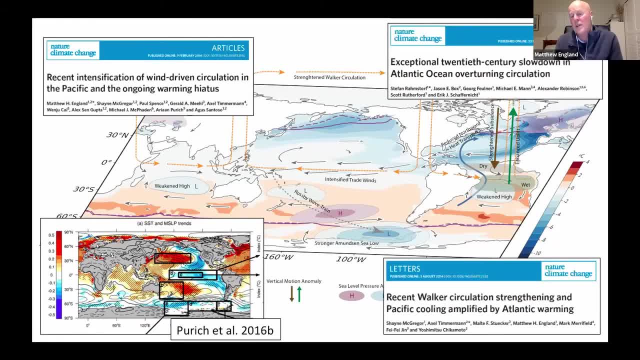 positive, though, frankly, for those of you who've actually been on our research, we were running up into the importance for the global scale teleconnexion emanating out of the north atlantic and the kind of um the so called, And the coincidence of over the last three or four decades we've seen each of these bits of the climate system change in this way, but nobody's put this together in a sort of coherent story yet that the Atlantic overturning circulation has very strong evidence of a slowdown. 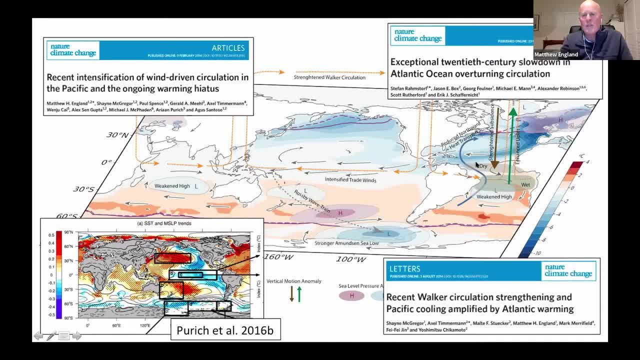 We've seen the tropical Atlantic warming and we've seen an acceleration of these trade winds and also the steepening of the atmosphere. low and so it's. it's a change in the system driven by climate change, but it's a change that manifests in in in teleconnections. 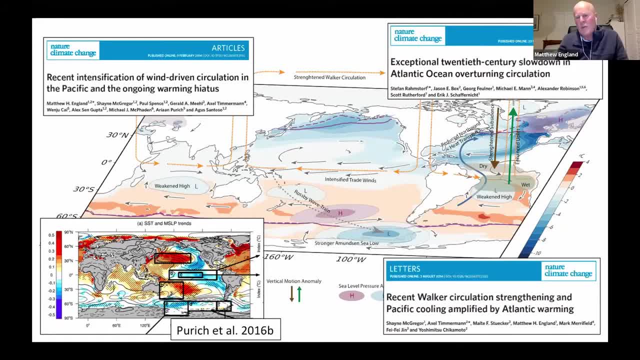 that reach from one hemisphere to the other, right across the tropics, and links really all of the changes originating from the from the Greenland meltwater entering the the North Atlantic Ocean. Okay, Juan, how am I going for time? 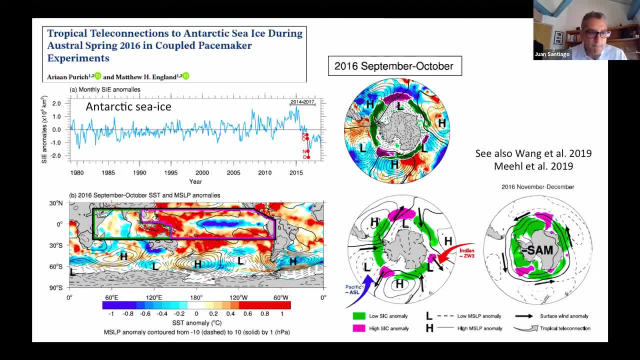 Yeah, you've got about five minutes left. Thank you so much. Okay, so in the last five minutes I want to talk a little bit about the southern hemisphere and in particular I spoke a bit about teleconnections from the tropics to high latitudes. I want to talk to you a little bit about a discovery we just made, in the last year or so, that we're very 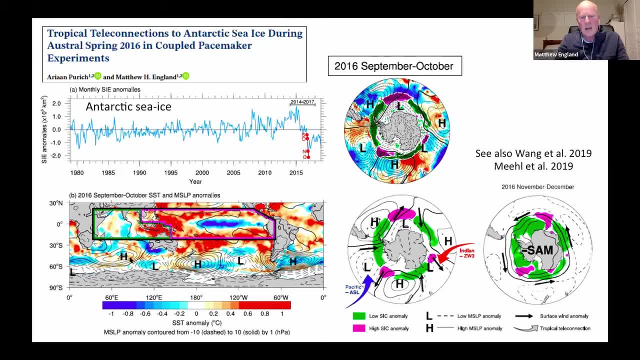 excited about Because it leads to a deeper understanding of this pattern of pressure systems. you get across the southern ocean and we talked about this as a zonal wave three pattern, and what we mean by that is you have typically in any given snapshot of the atmosphere in the southern hemisphere- is a pattern of three high pressure systems and three low pressure systems alternating between each other. 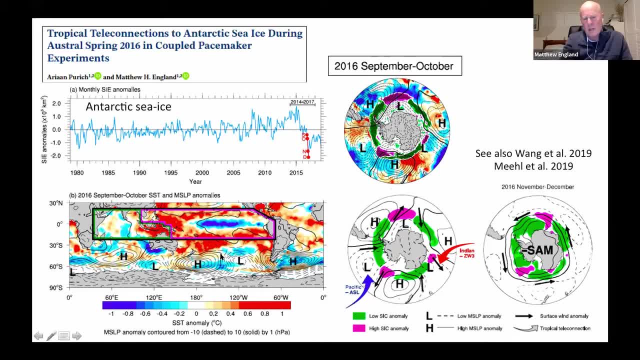 Now, as you can imagine, these pressure systems are associated with very strong north- south flow, And so you either bring- And so you either bring- warm air towards Antarctica or cold air moving back northwards and this huge sea ice decline that occurred in in the recent years. so Antarctic sea ice was gradually increasing and confusing climate scientists, although we worked out why that was occurring, due to a bunch of processes, but this collapse caught everybody off guard. 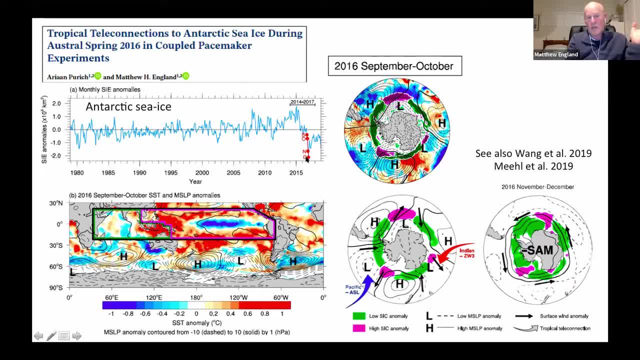 And it turns out that it actually got to levels that we had never seen in the observed record. so this decline was dramatic And it was due to this sort of wave number three pattern. It actually became very, very strong for a couple of months. 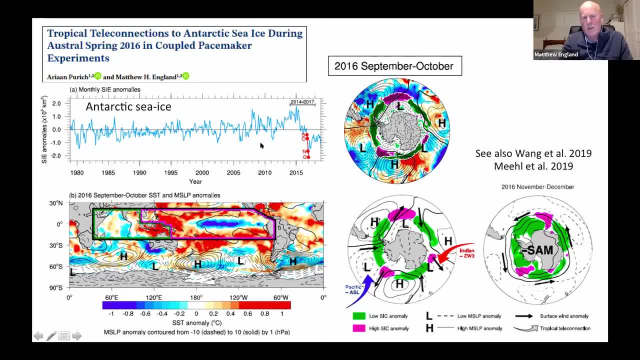 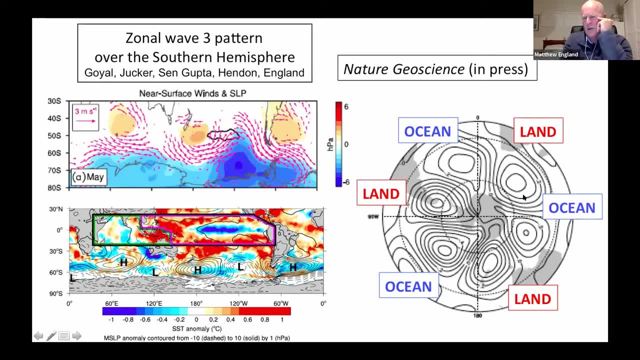 So it actually wasn't like all of our topics. he has declined. it's actually there was sort of hotspots of decline that coincided with these warm air masses moving towards Antarctica, and so We showed this link in this paper. we showed this link back to the, the tropical Indian Ocean. 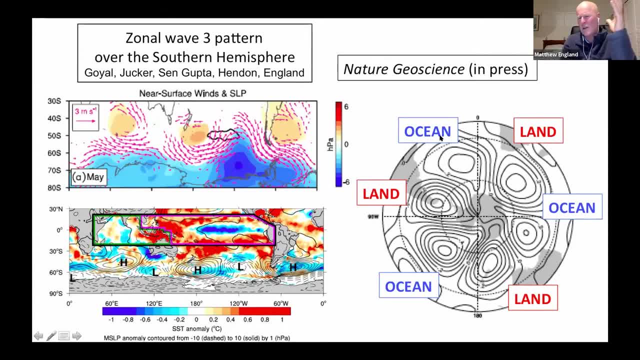 But we went into a deeper dive With this To, because it's sort of quasi-stationary um. it was thought to be linked to this land ocean geometry and so, with the southern hemisphere wave three pattern being so strong, the sort of assumption, if you like, was that the fact we have three masses of land and three bodies of ocean alternating. 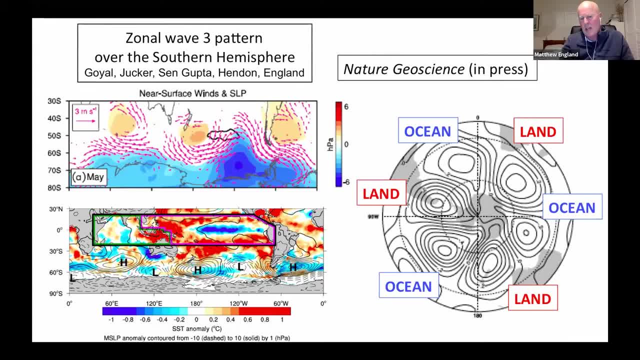 their position around the southern hemisphere that this gave and and these- the ocean and land surface- do have very different interactions with the atmosphere above, and so it's kind of plausible that you might think that the continental configuration gave rise to this three-wave number pattern. but one of my grad students, Rishabh Goyal, is just about to finish up and submit. he's 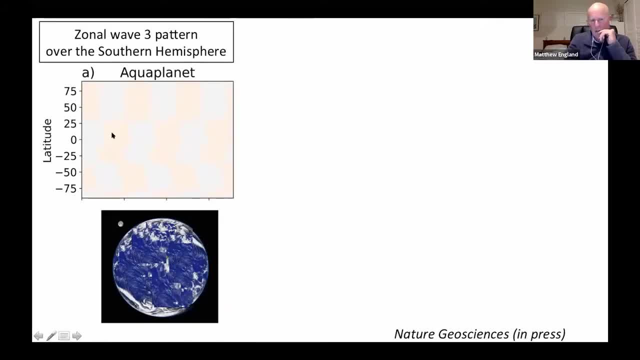 done a great job with his thesis and and one of the things we set off to do to start with is to sort of build up our planet, if you like, in the model, build up the planet of earth from a very simple aqua planet system and, excuse me, progressively add these land masses to see. 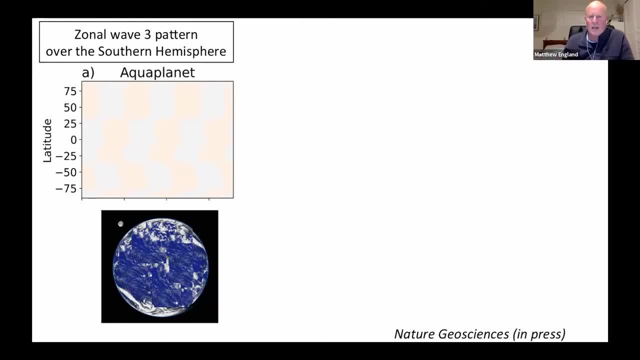 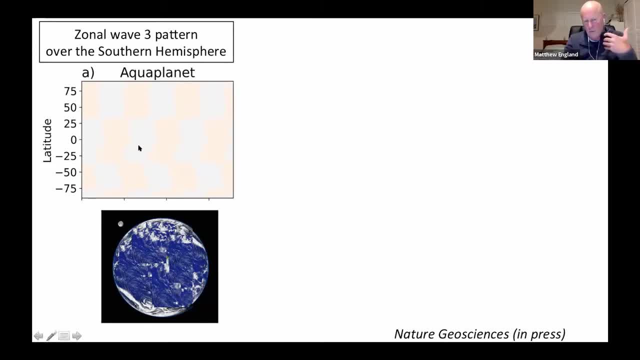 and at the top here is, is the Fourier filter to pick out the the wave number three pattern, that that comes about from each of these simulations, and I'll only show you three of these. one is the full aqua planet. the second is where we just have land masses, as you can see here. 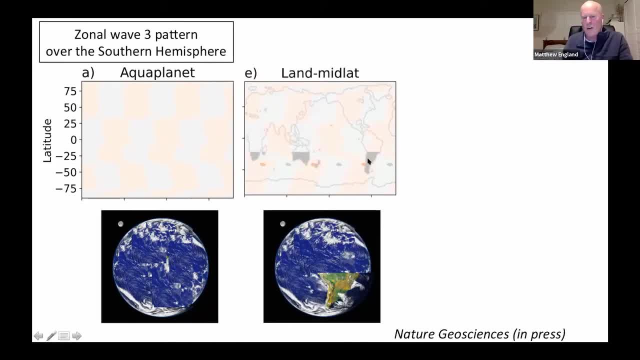 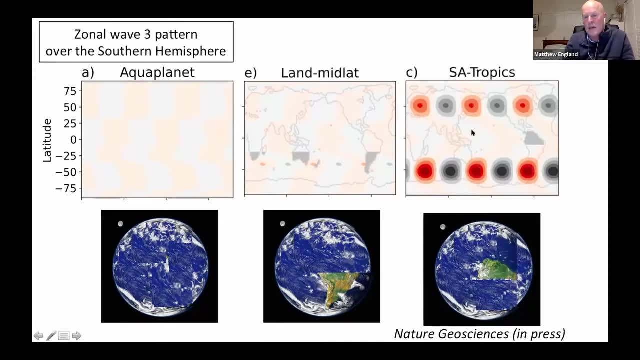 in the gray, at the mid latitudes, where they occur in the southern hemisphere. and the third case is just a a single piece of land over South America. it could have been any piece of land over the tropics- it's a fully aqua planet system in this third case- but we just have a single piece of land here to trigger. 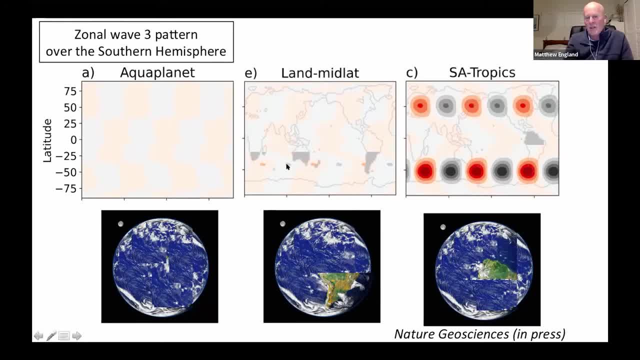 atmospheric convection and what we found is that actually the land masses in the southern hemisphere really did nothing to generate a wave three pattern. so this assumption that had been around for 30 or 40 years was was a simple one. it hadn't been tested. it turned out to be wrong. 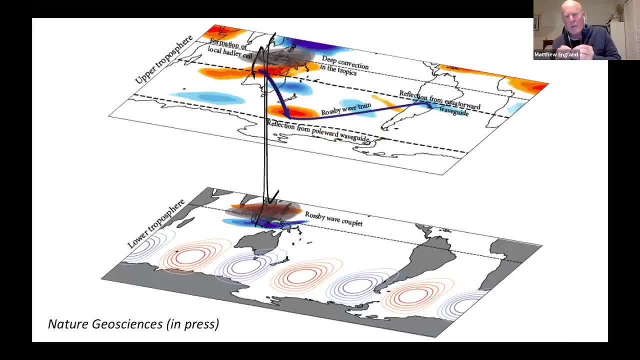 and instead of instead of the wave three pattern being there due to land masses, it's convection in the atmosphere, so it's a the rising of air over warm water in the, in the tropics, that generates this disturbance that propagates poleward and then, once it propagates poleward, at these latitudes there's a very strong, uh westerly wind. 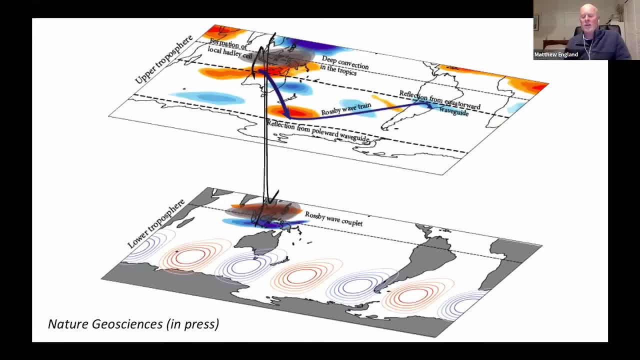 jet that propagates from west to east, and and the Rossby waves that i spoke about. if you look at their dispersion relationship, they propagate westward and you get. you get a whole bunch of waves, not just wave three, you get wave numbers um one through to six, seven in the system, but it's 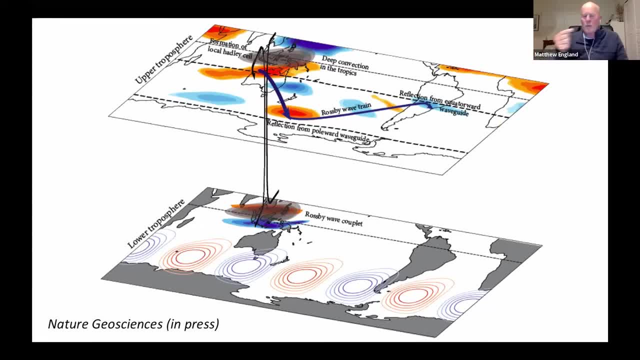 it's this wave three pattern that has a phase propagation going upstream against the dominant atmospheric circulation, going the opposite direction. that gives you a standing wave three pattern and, as we know from this, the northern hemisphere. when you have these standing waves in your jet stream, it can lead to 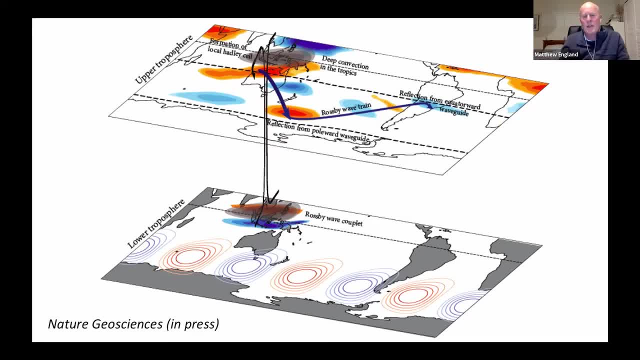 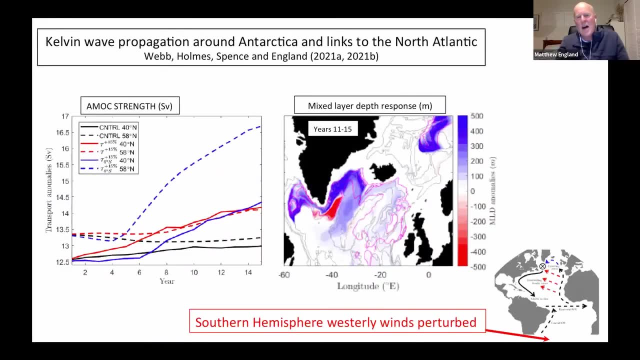 these very extreme um weather, weather events over the northern hemisphere, and so that's where i should finish up. i had another story that takes us back from the southern ocean back to the north atlantic. um, but i sense i'm probably that one's been generous with time and i've probably got 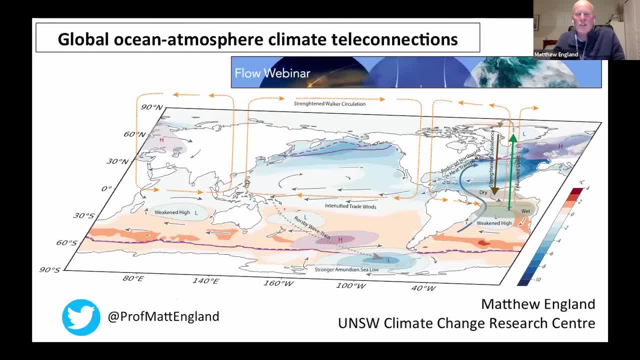 the stage where i should um wrap up there and thank you for tuning in and answer any questions, if there are any. thanks, thanks a lot, uh, matthew, that that was great. um, okay, well, let me start by saying: matt, a nice talk and particularly nice slides, uh, the bed behind you, i'm surprised you're. 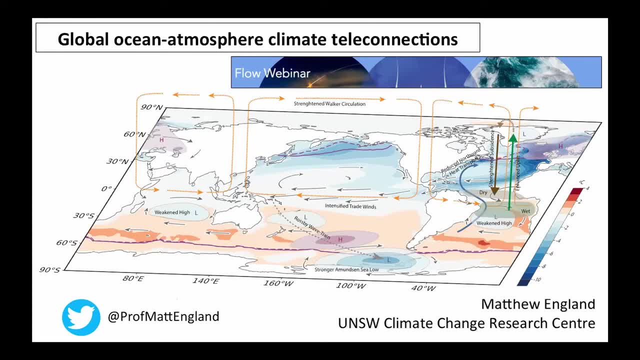 not in it, it's about 1: 30 in the morning. uh, most impressive. but what i wanted to ask you, you, what do you think the next big fundamental step forward is to have us understand the climate better. ah, yeah, it's a good question, her, but i and i- i think i mean the atmospheric scientists- are 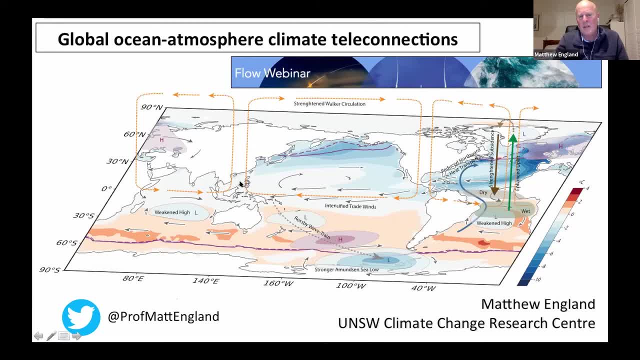 talking a lot about this convection in the tropics um the. the our measurements of of tropical convection is is there. it's a tough thing to measure. it happens on very fast time scales and, as you know, the the velocities involved are rapid and it's tough to get in there and make measurements. 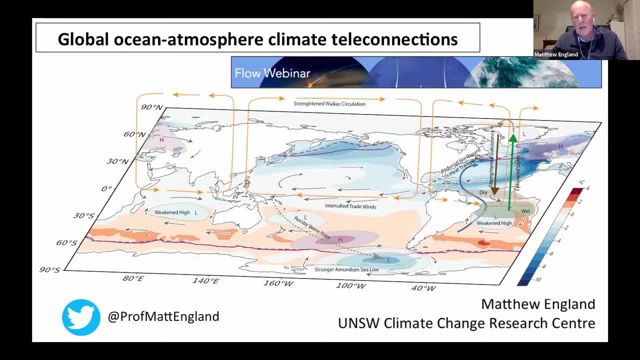 and the models we have don't do that physics terribly well. um, for the ocean, we keep building models with higher resolution and we- we don't, as you know from your work, we haven't yet found the limit of kinetic energy in in the system. what i mean by that is every time we build more resolution in these. 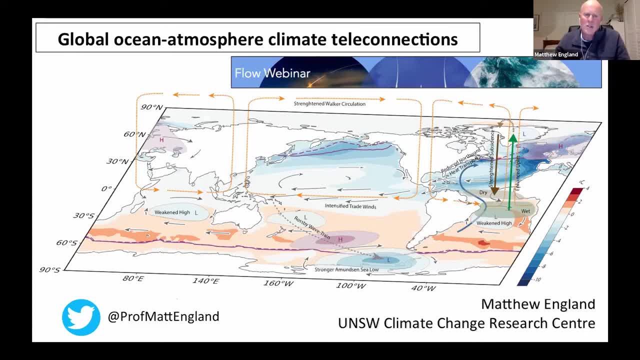 models, we, we haven't saturated kinetic energy and so um. it's kind of a boring answer to give, but i think these finer scales that we still haven't tapped into in these simulations, the submissive scale um is the next frontier in these models, and so um, you know, i think the next frontier is to. 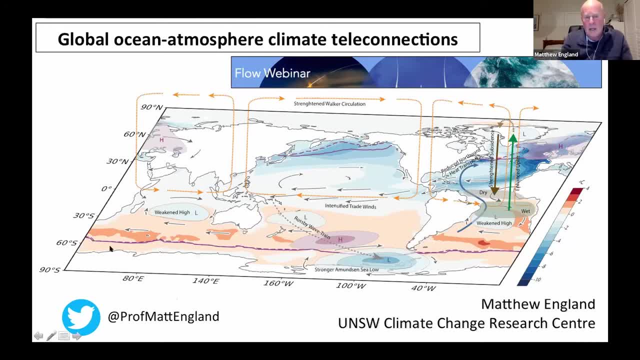 And one of the areas I'm interested in at the moment is the intrusion of warm water around the Antarctic continent And down there the Rossby radius really gets so fine that we need a resolution of hundreds of meters And the typical global models we use. 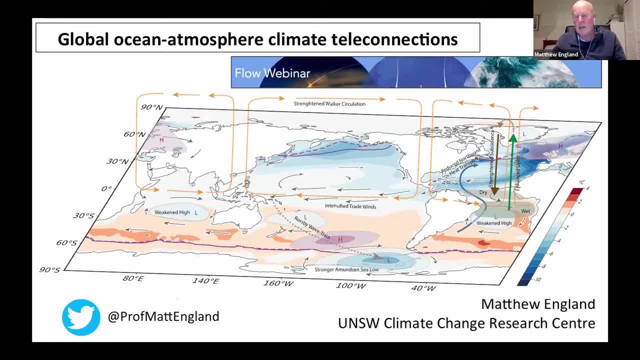 for climate projections have resolutions down there of at least 10 kilometers, but typically even more than that, And so to me it's that age old answer we've given for a long time. It's those submissive scales that we don't get to with these models. 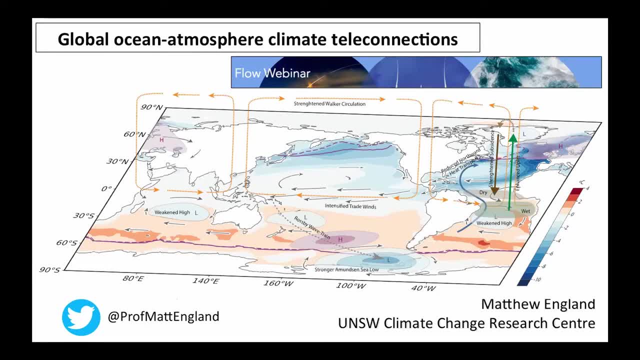 Matt, very interesting presentation. I was just wondering if you could give us a little bit of insight into the types of computer systems, computer hardware, that you use for running these simulations, and what's the scale of actually doing simulations of this sort. Yeah, no, we dominate the use. 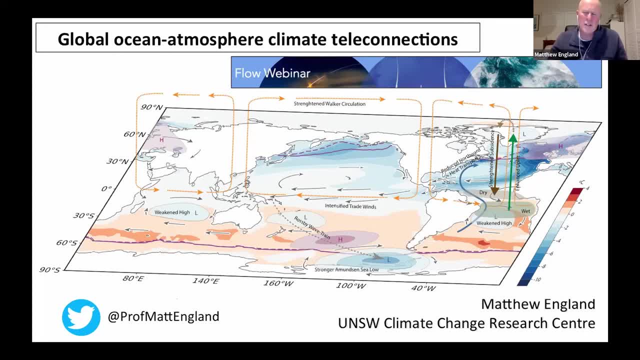 of our national supercomputer here in Australia And I'm not good on the specs of the computing systems we use. I've got to declare that upfront. I chew through the hours and I have. we have petabytes of data on these systems. 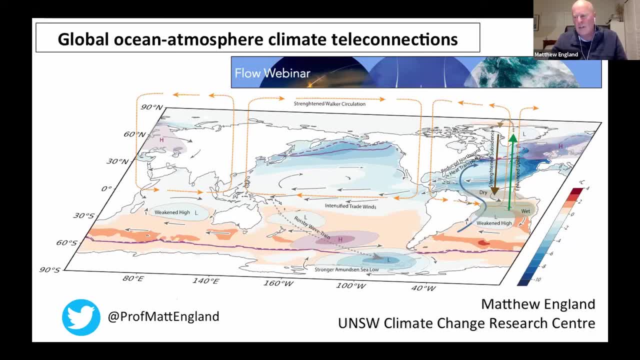 but the actual specs I don't have handy, But I think the system we use here in Australia is one of the top 20 in the world, top 30 in the world. But you're right, it's a good question because we do have a huge need for computational resources. 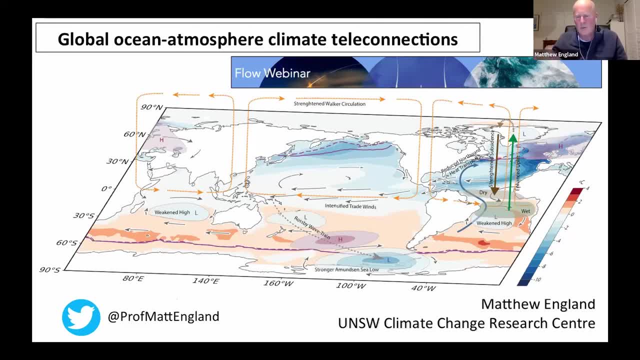 And we build models that push the limits of those resources, both in terms of the computational time and the memory, the memory processing and the storage they use. So that's been how we get to more. resolution is not the limit. is the computing system was we use?